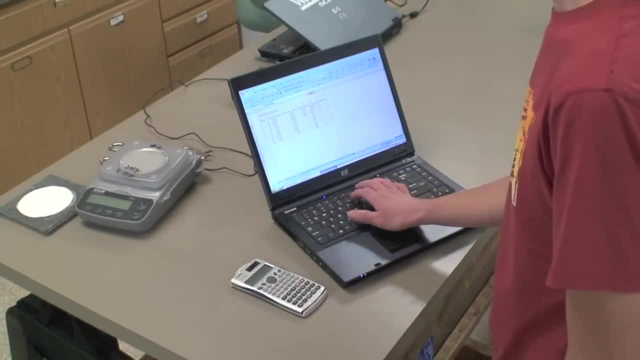 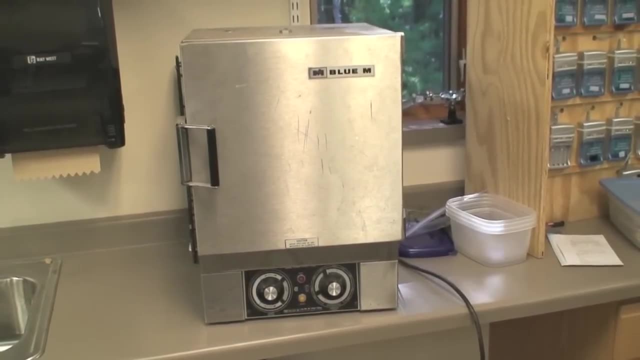 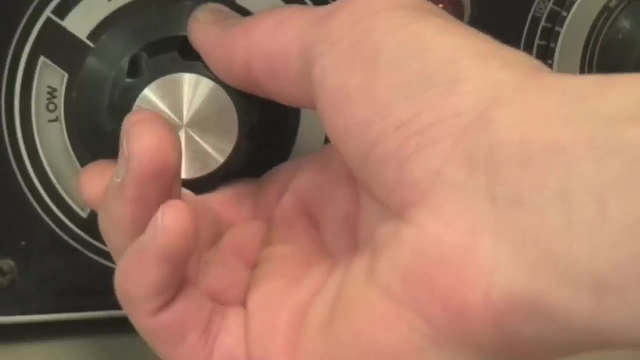 Do this for each crucible containing soil and enter these weights into your data table, noting that the soil is wet. To dry the soil, you can use a special drying oven. Set the power control to medium. The temperature should be set to 125 degrees Celsius. 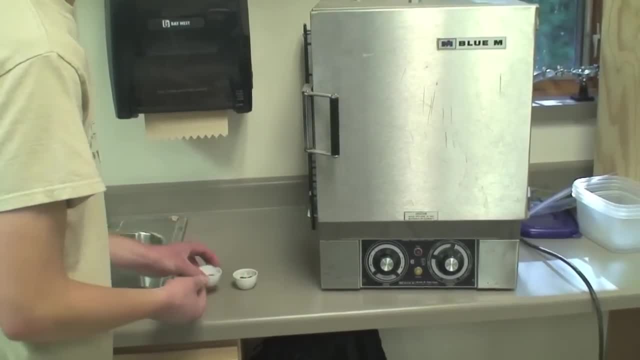 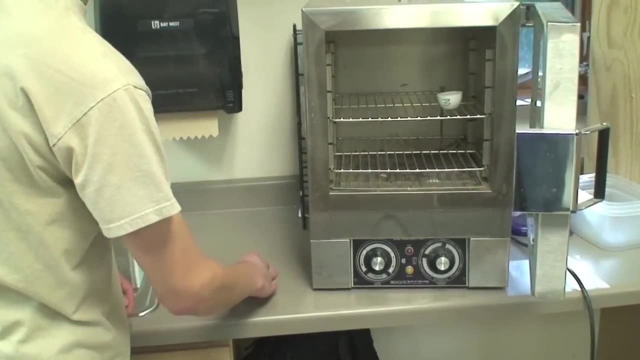 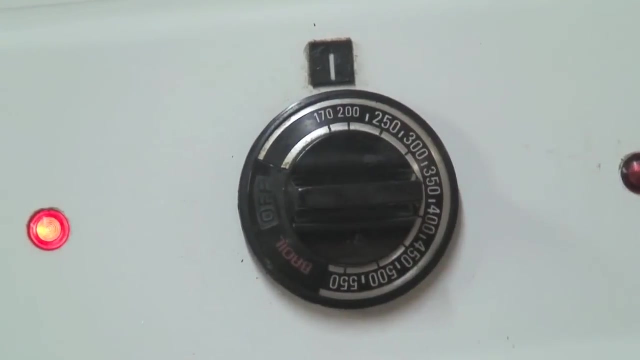 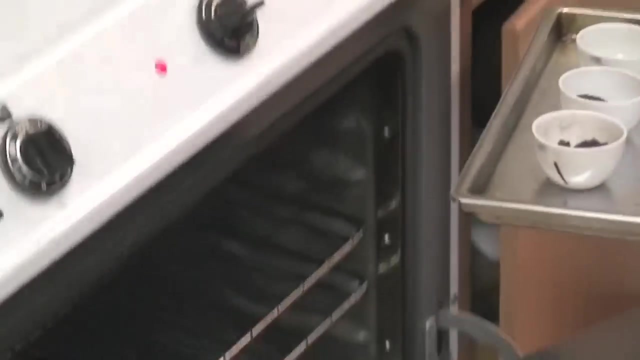 Put the crucibles into the drying oven and let the soil dry over night. If you don't have a drying oven, you can use a kitchen oven set to 200 degrees Fahrenheit. Put each of your crucibles on some kind of pan or sheet and leave them in over night. 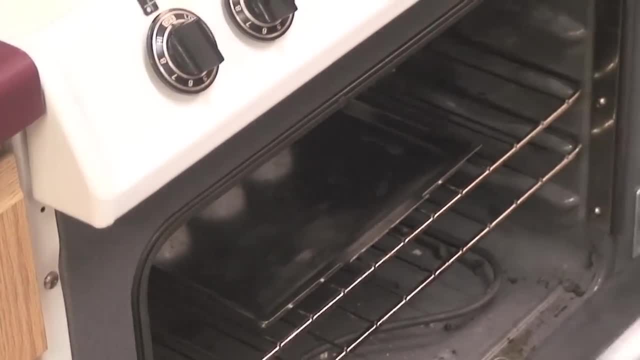 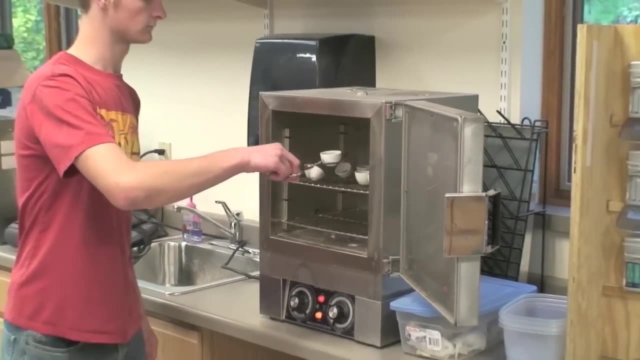 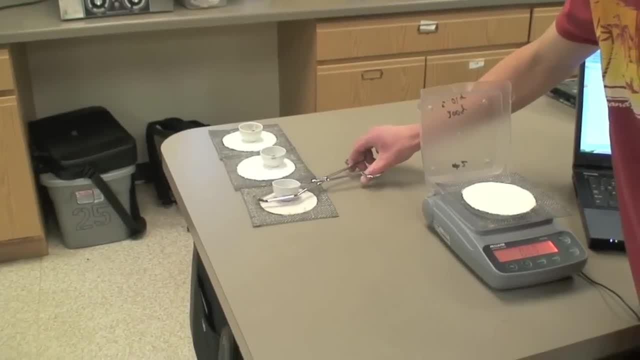 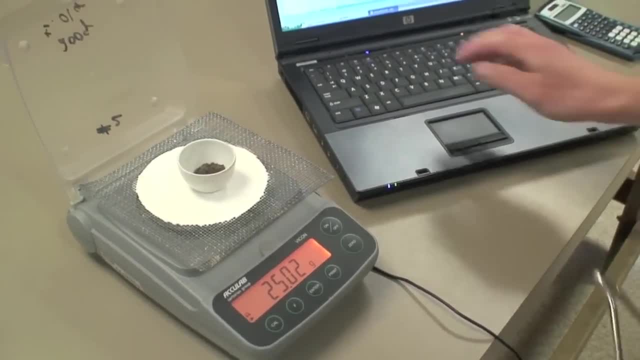 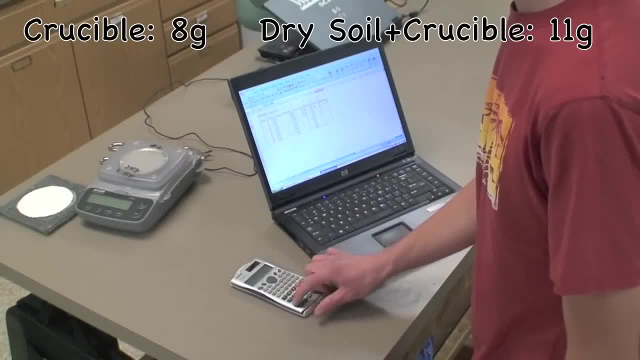 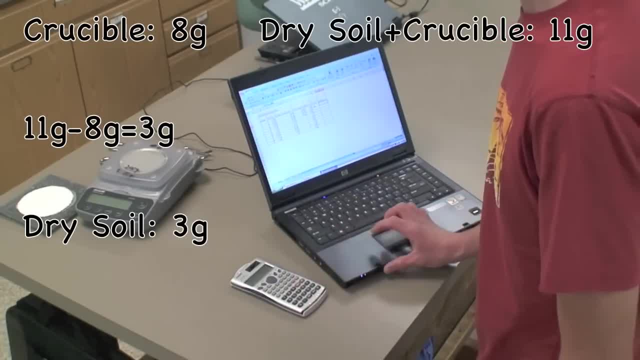 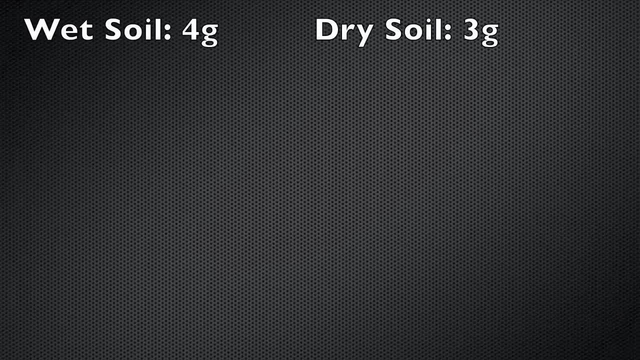 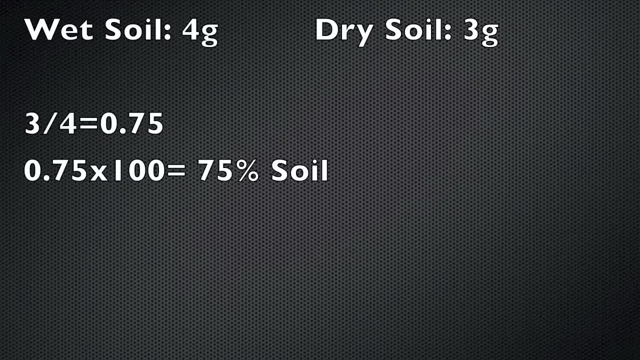